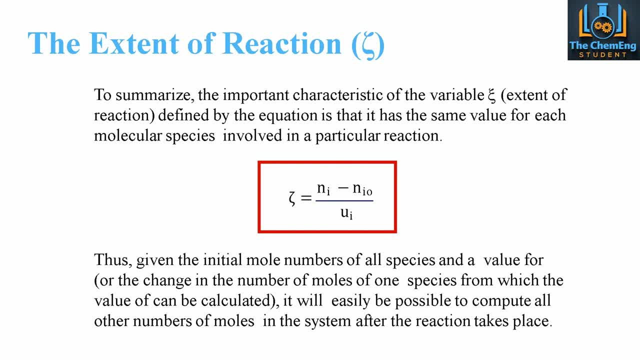 always do, is it always moles that can be related to each other? So, for example, if we had A plus B goes to C plus D and we'll say that this is 2 here and this is 3 here. Now these stoichiometric coefficients are in theory. these are the 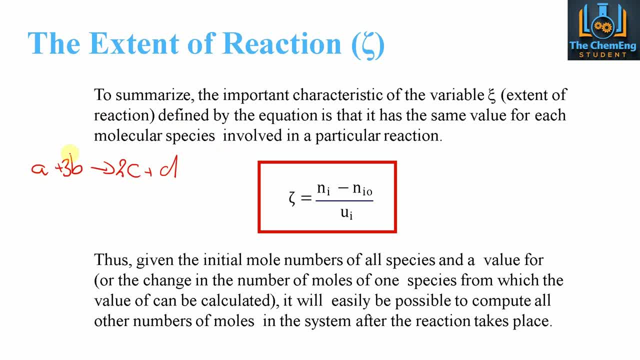 ideal scenarios. So that means that one mole of A plus three moles of B would produce two moles of C and one mole of D. Now this is moles. that binds all these together. We can't use mass to bind these together, because the mass of the each 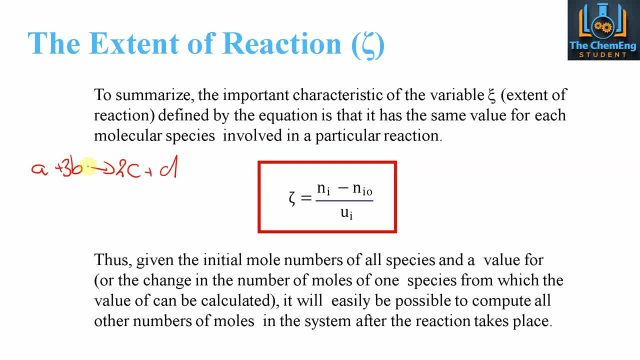 species, for one mole will be completely different. So you can see that in the GFM values in the chemistry data booklet or the grand formula mass of different compounds. So by expressing the values in terms of moles it makes it easy to determine the actual number of moles we have within the system, both as reactants. 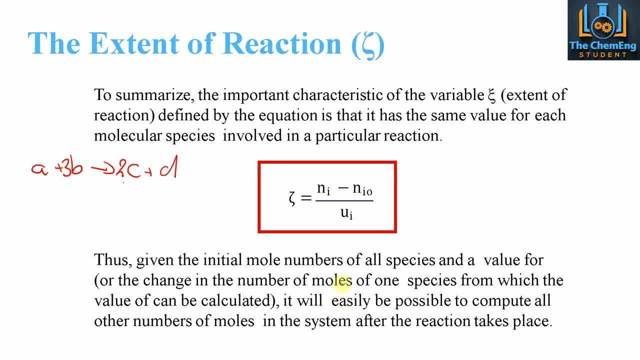 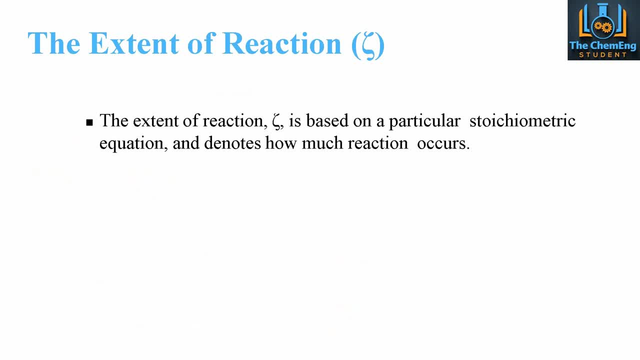 and as products. So that's why it's very, very important that it is in terms of moles. Now, the extent of the reaction is based on a particular stoichiometric equation and it denotes how much reaction actually occurs. Now the units would be moles reacting. So we're essentially saying that this value is 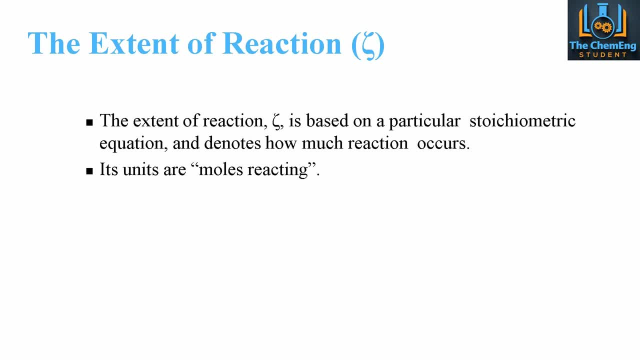 how many moles of the system has actually reacted. And the extent of the reaction can be calculated by the change in the number of moles of a species that occur, and then divided by its stoichiometric coefficient that we've seen in the previous slide. Now, for example, here, if we consider the 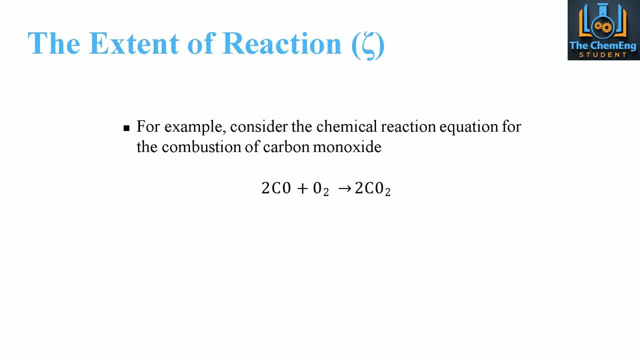 chemical rate equation for the combustion of carbon monoxide, then the signs of the stoichiometric coefficient to be used will confirm to what the standard practice in calculating the extent of the reaction would be, Namely that the products would have a positive sign and the reactants have a negative. 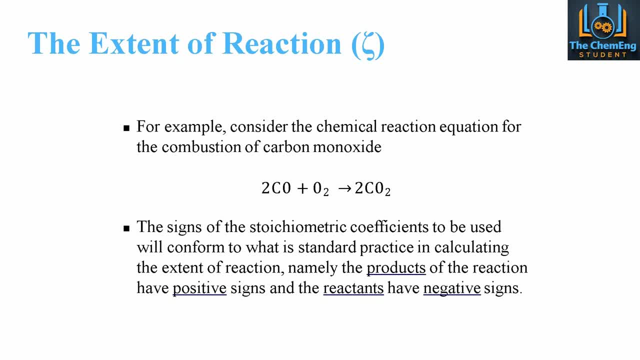 Now that features all throughout mass and energy balances in chemical engineering and also equates to a lot of the other equations that we see That when we talk about the reactant we tend to associate that with a negative, and when we talk about the product we 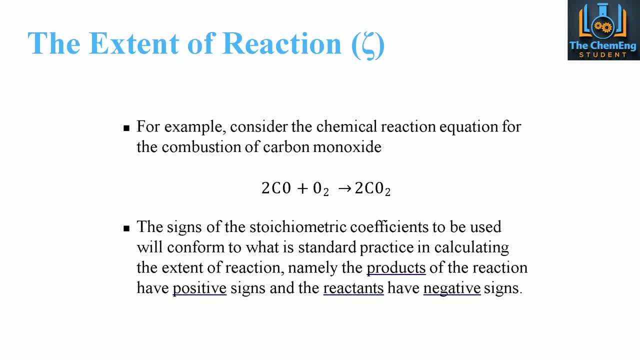 tend to associate that with a positive. now what we're seeing here is that if we have say, for example, for the co2, then if we have the initial amount of moles of co2 with, say, 0.5, and then the final number of moles would be 0.25, then the extent of the reaction would be that it would be. 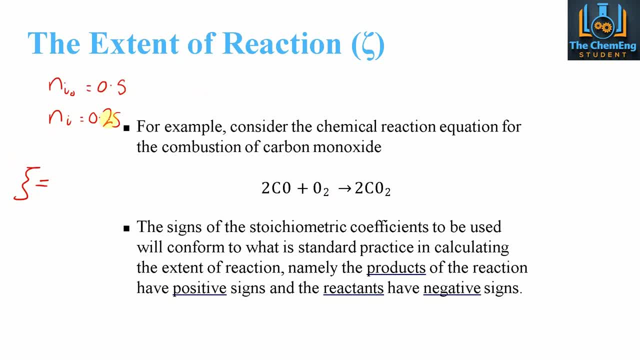 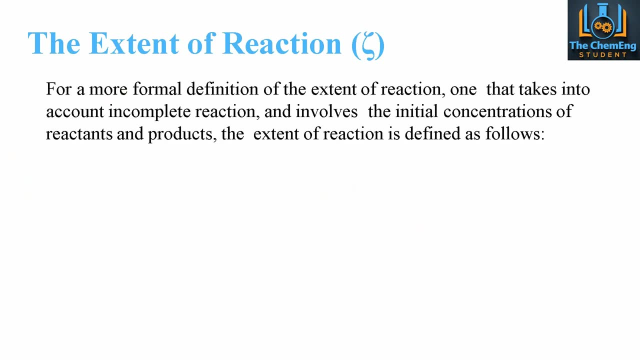 the initial, it'd be the change in these values divided by the stoichiometric coefficient here of 2, and that would then allow us to equate the corresponding values for the other components. so the more formal definition and the more formal definition, and the more formal definition and the more formal definition. 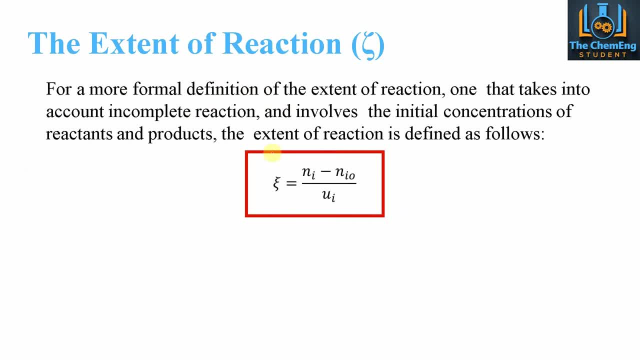 it's the same equation that we've seen, but the more formal definition would be that is based on the initial concentrations of the reactants and the products. so ni here is the number of moles of the species after the reaction has occurred. so in the previous example that we 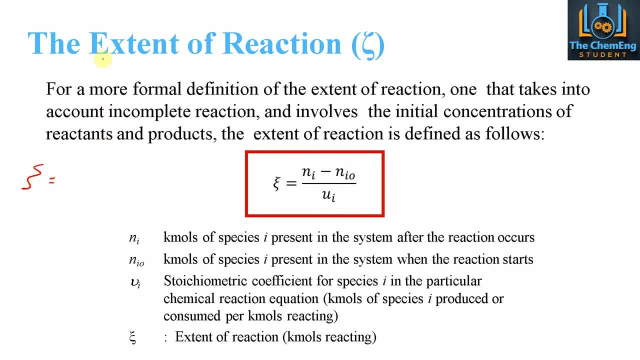 said so for zeta. if it was, we say 0.25, then it would be minus and then it would be zero, point y. three plus 0.5 divided by two, because ni is a species at the beginning, when the reaction starts, and then the stoichiometric coefficient is the value at the start of the 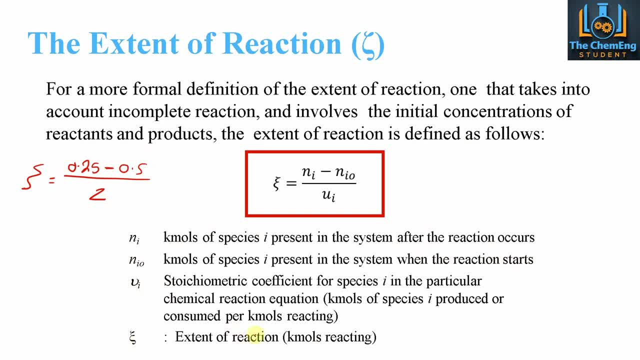 chemicals, and then zeta, of course, is the extent of the reaction and for this case, kilomoles reacting. so you would carry this calculation out and get the value of zeta. now you can see that the reason we get a for the reactants is because this would be a negative quantity. However, if we look at a, 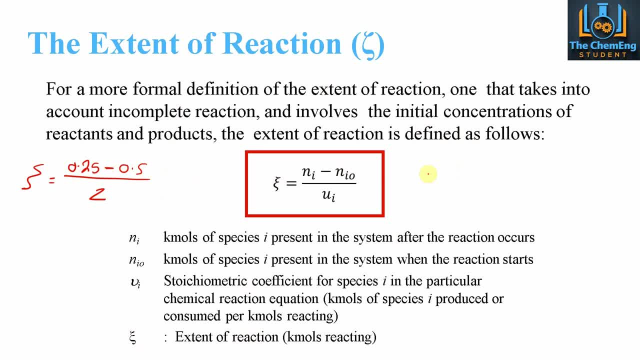 positive quantity, ie a product. then our zeta would become, say, for example, we had the production of water. Then at the beginning, say our initial moles, Ni naught was zero, and then Ni final was say 5. Then what we would have is it would be 5 minus 0 over say 2. Then we have